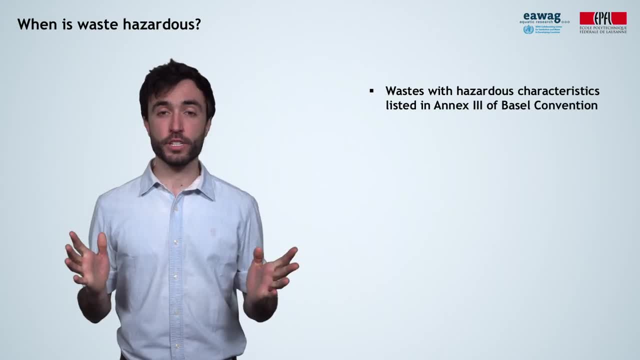 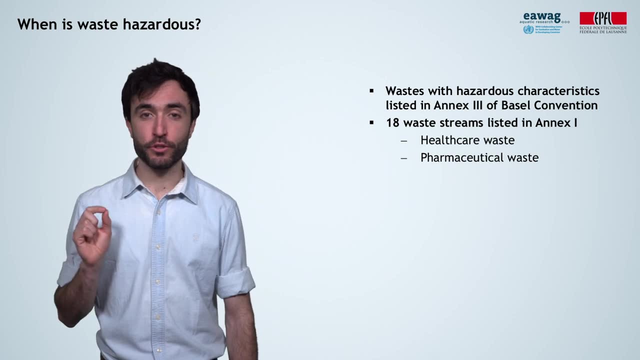 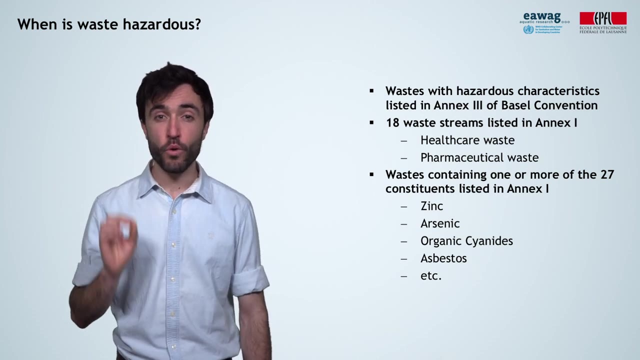 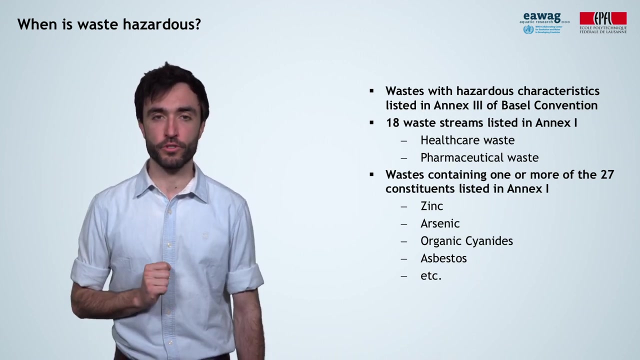 and corrosive. All these characteristics are explained in Annex III of the Convention. Besides, there are 18 waste streams and 27 constituents, such as zinc, arsenic and asbestos. they do not possess any of the previous hazardous characteristics. Finally, the Convention 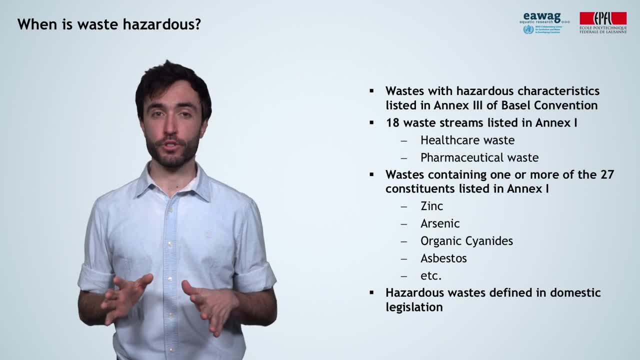 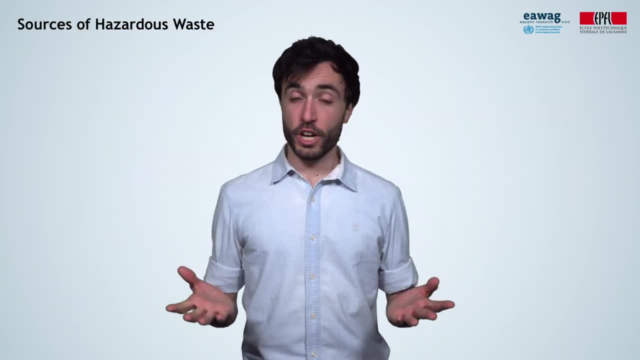 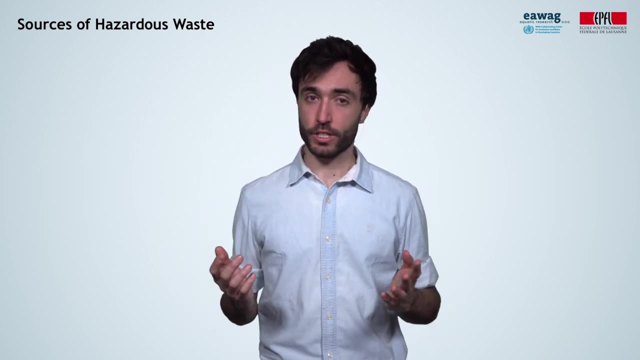 also states that wastes that are defined as hazardous in the domestic legislation of a country should also be considered as hazardous. So who generates, and where is hazardous waste generated? Well, obviously, hazardous waste arises from multiple sources. Industries are the biggest hazardous waste generators In most countries, however, hazardous waste is. 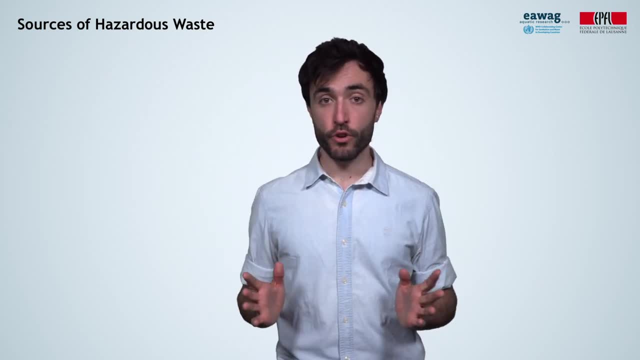 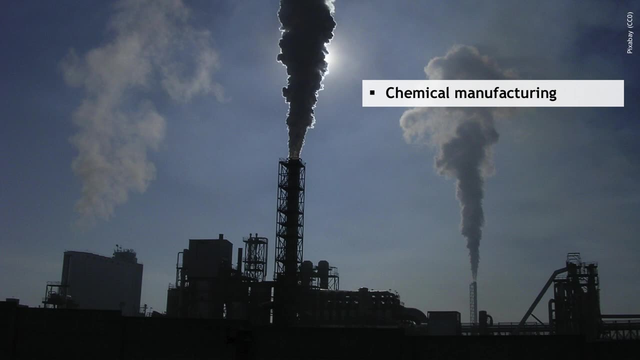 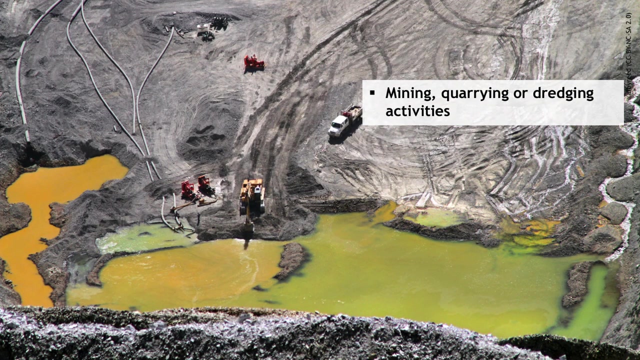 generated by the government. However, they are responsible for managing their own wastes and therefore their waste does not enter the municipal solid waste stream. Important generating sectors are the chemical manufacturing, the petroleum and coal product manufacturing, mining, quarrying and dredging activities, the pulp and paper industries, wood remanufacturing. 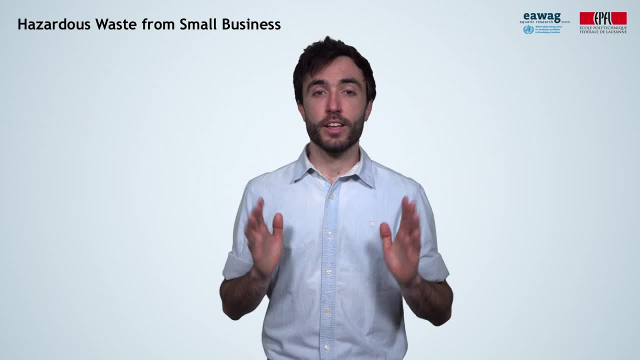 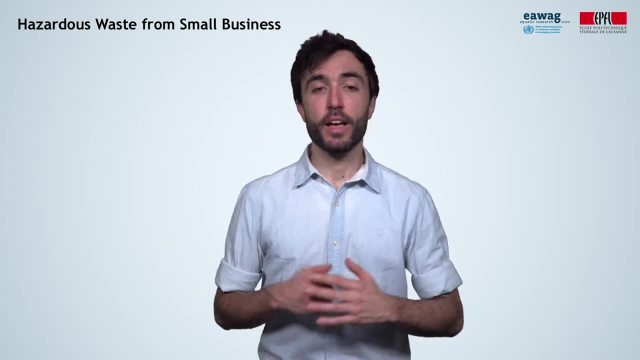 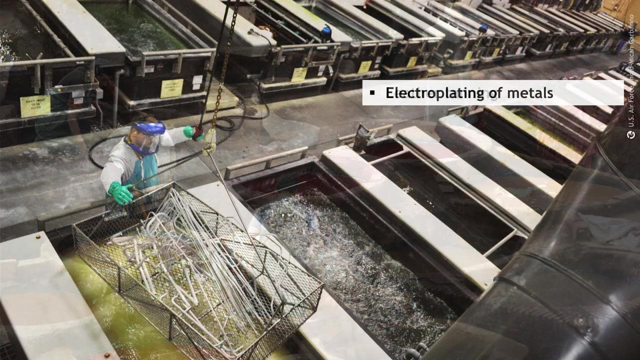 facilities and the pharmaceutical industry. Small-scale businesses can also generate hazardous wastes, which might be part of the production of hazardous wastes, The municipal solid waste stream. Examples of such businesses are car workshops, leather tanning enterprises, electroplating shops, photo finishing shops, construction and demolition. 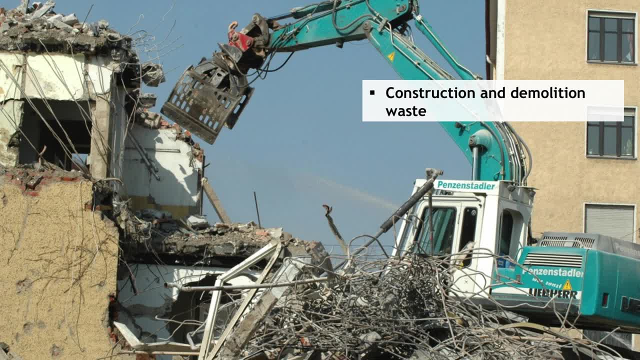 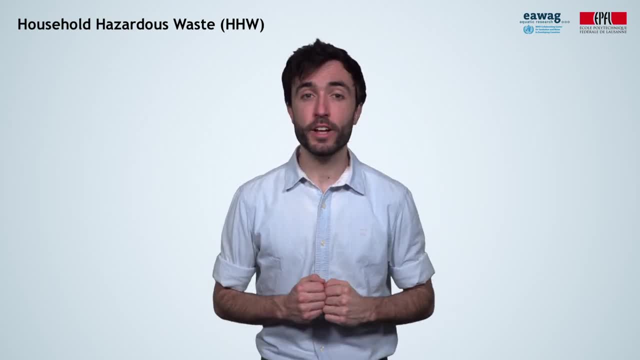 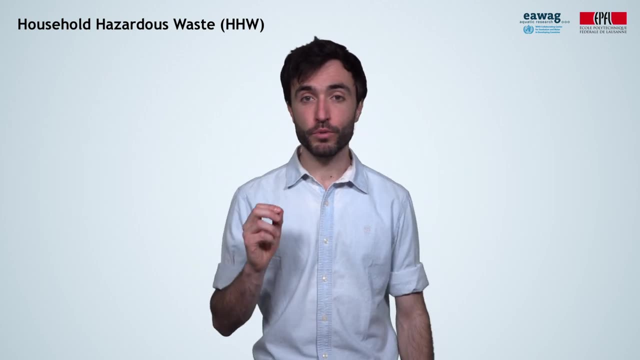 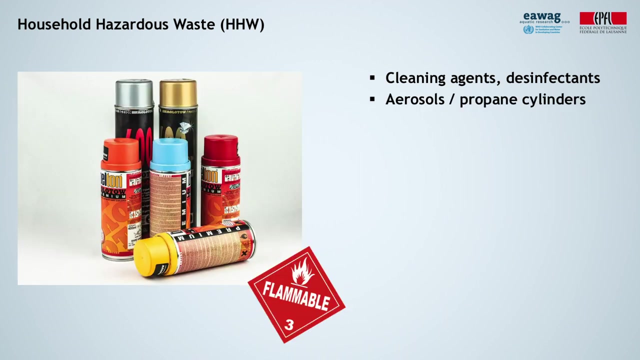 companies that produce wastes containing asbestos, etc. Household hazardous waste. I bet that many of you are not aware of how many everyday items are hazardous or contain hazardous materials. Let's explore some common examples and the possible hazards they can pose: Cleaning agents and disinfectants, aerosols, propane cylinders, batteries, cosmetics, such. 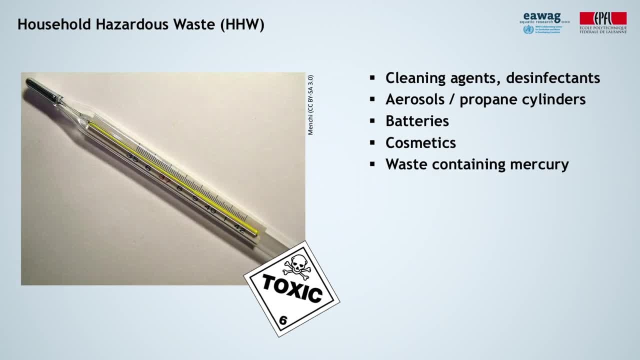 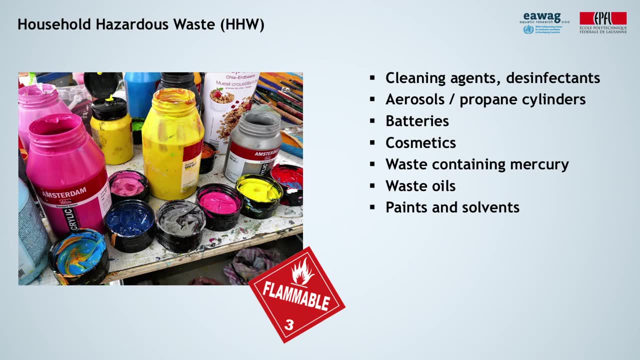 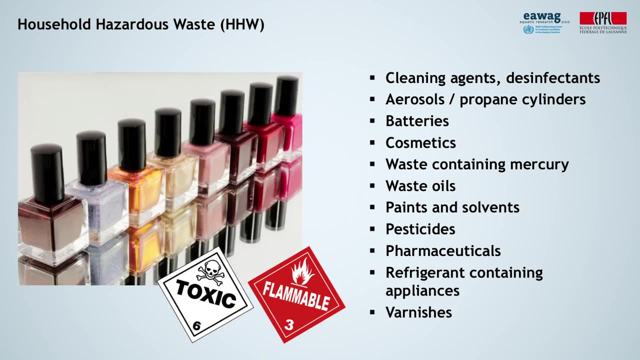 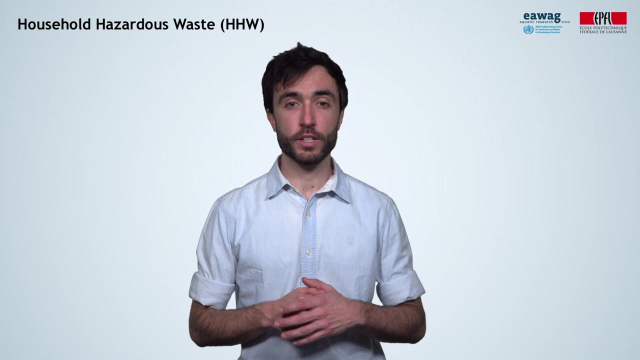 as hair dyes. waste products containing mercury, such as thermometers or fluorescent lightening. waste oils, paints and solvents, pesticides, pharmaceuticals, refrigerant-containing appliances, varnishes. The share of household hazardous waste over the total municipal solid waste on a global. 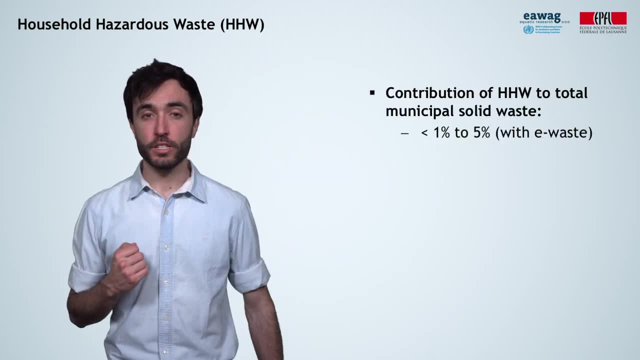 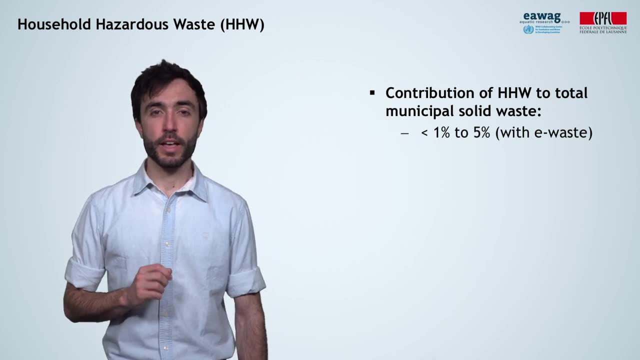 basis is unavailable. However, estimates suggest less than 1%, but up to 5% if e-waste is included. In spite of this relatively low share, its impact should not be neglected. As a side note, the parties of the Basel Convention, together with governments, municipalities. 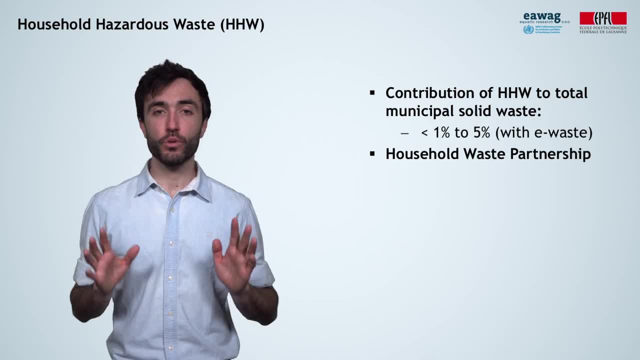 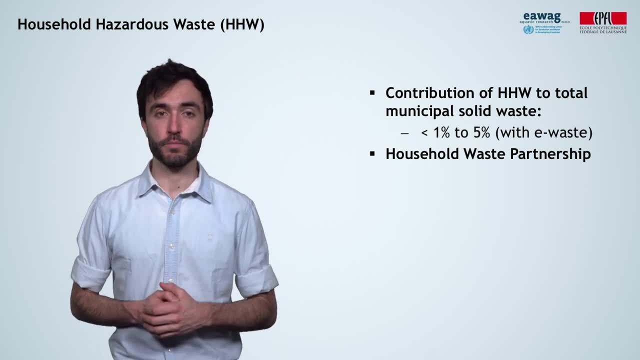 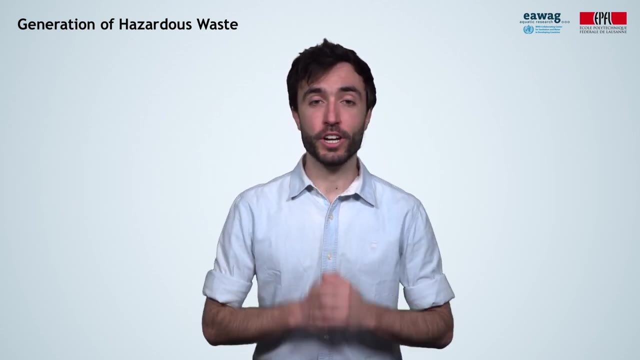 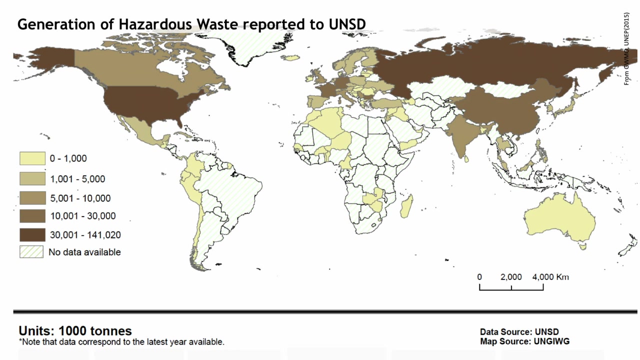 and industry have set the so-called Household Waste Partnership with the objective of providing guidance on the environmentally sound management of household waste. Now that we know what hazardous waste is, let's have a look at how much we generate worldwide. This map shows the amounts of hazardous waste generated per year and reported to the United. 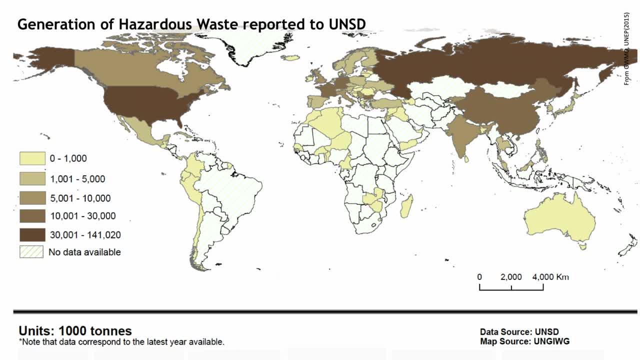 Nations Statistical Division in 2009.. This map shows the amounts of hazardous waste generated per year and reported to the United Nations Statistical Division in 2009.. Notice that there is no data for many countries and be aware that the amounts reported are most likely underestimates. 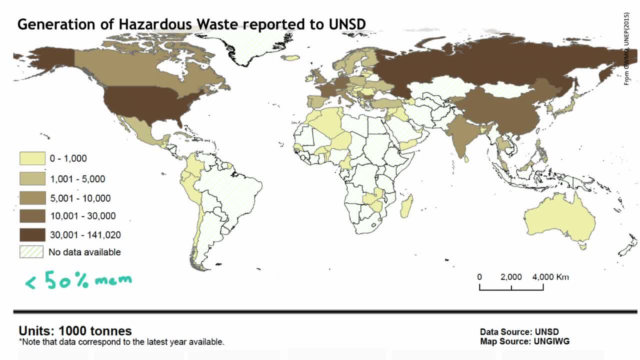 Unfortunately, fewer than 50% of the countries taking part in the Basel Convention report hazardous waste generation, import and export data. However, from those who do report, it can be estimated that at least 10 million metric tons of hazardous waste have been crossing international borders over the last 10 years. 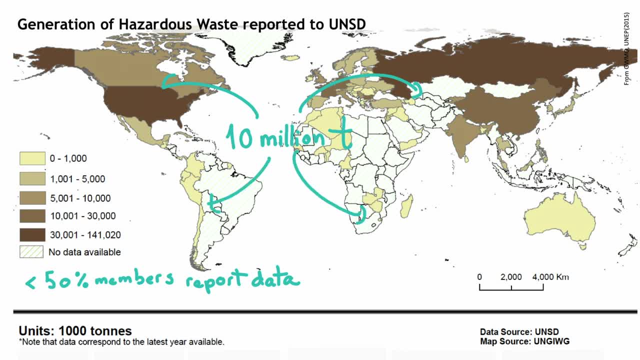 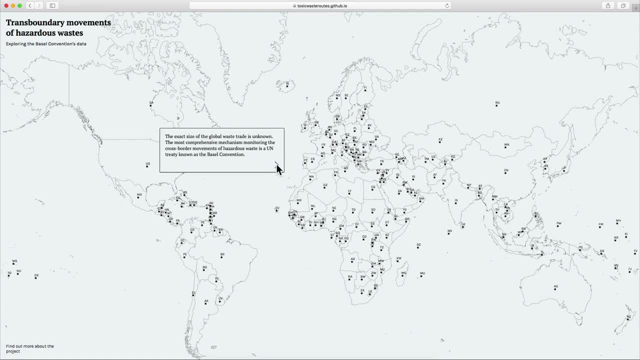 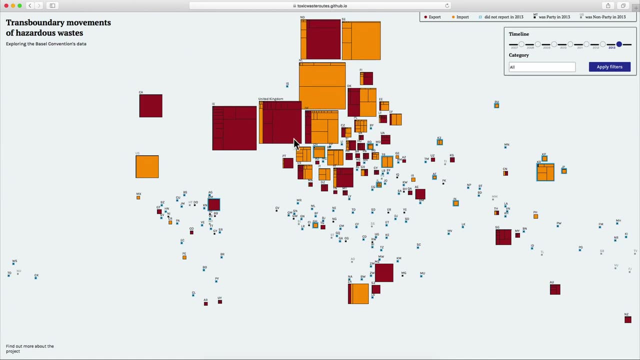 This is a significant number. Toxic Waste Routes is an interesting project which tries to visualize these imports and exports in an interactive tool. By clicking on the top of a country, Germany for instance, we see the amounts of hazardous waste exported in red and imported in clear orange. 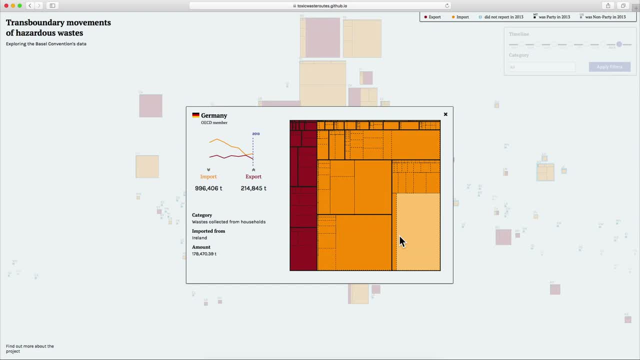 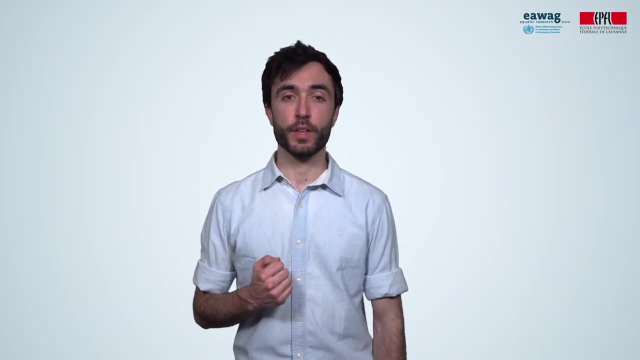 Each box represents an importing or exporting partner country and by putting your cursor on top you can see the amounts of hazardous waste exported in red and imported in orange To get a more detailed information about the nature of waste and the specific amount. The management of hazardous waste has become a specialized discipline. 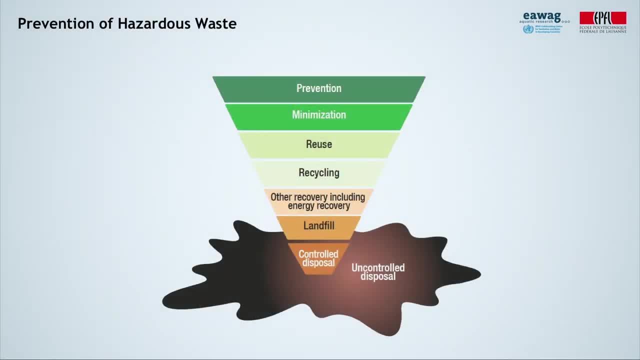 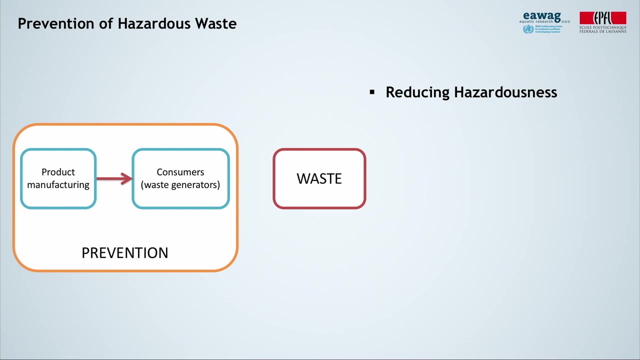 We will use this simplified diagram to explain the main concepts. We will refer to the waste hierarchy correspondingly. Let's start with prevention. This can be done by the product manufacturers by reducing hazardousness, for example, substituting toxic materials with less toxic waste. 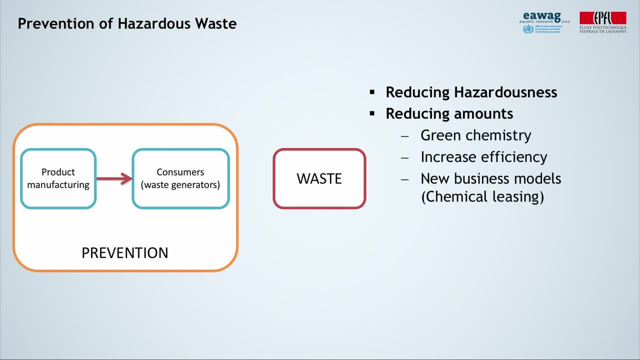 Let's start with prevention. This can be done by the product manufacturers by reducing hazardous waste- for example, substituting toxic materials with less toxic waste- and by reducing amounts, by modifying manufacturing processes to follow green chemistry, increasing efficiencies and establishing new business models, such as chemical leasing, which implies renting out instead of selling. 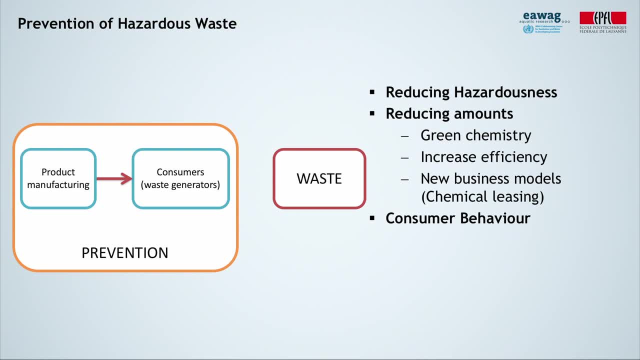 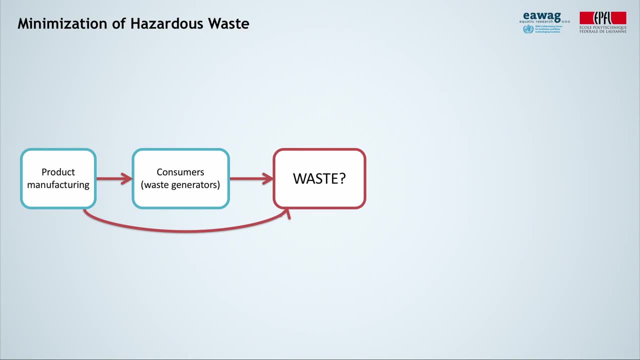 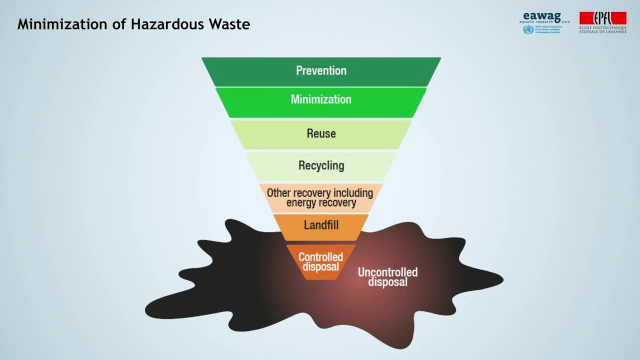 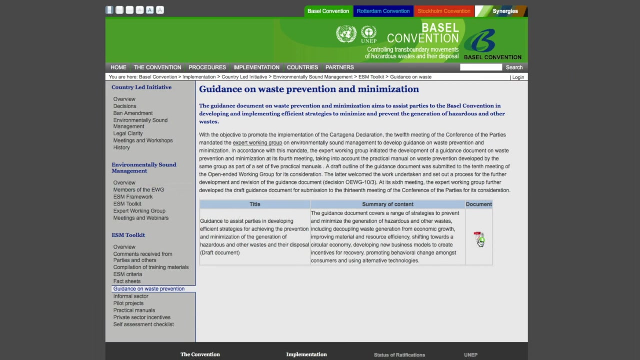 chemicals. Prevention can also be implemented by influencing consumers' behavior to choose products which, before the product turns into waste materials can be reused. This represents minimization of waste, the second layer of the hierarchy. Check for the term's guidance on waste prevention and minimization on the internet to get some. 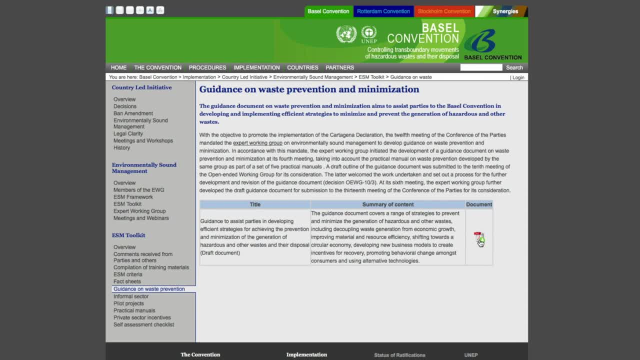 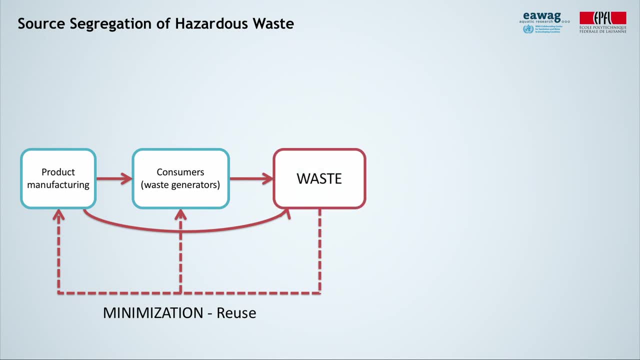 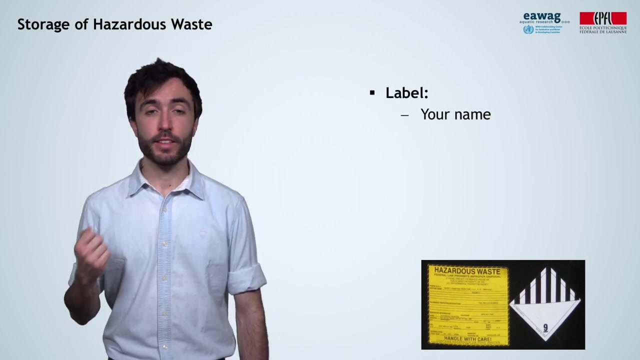 more insights on this issue. Then the materials we refer to as waste are generated. It is imperative to source, segregate all this waste, especially the hazardous waste. Then the waste needs to be stored. This can be done by using small containers. These containers should be labeled indicating your name, the 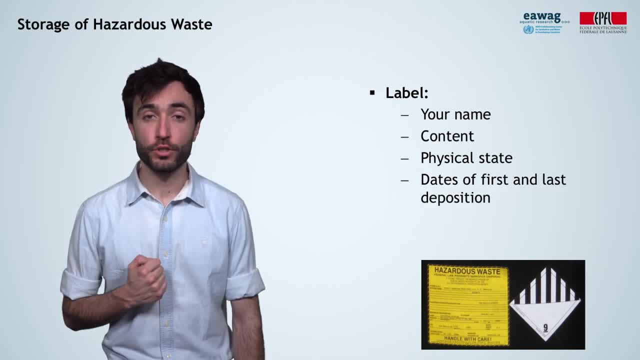 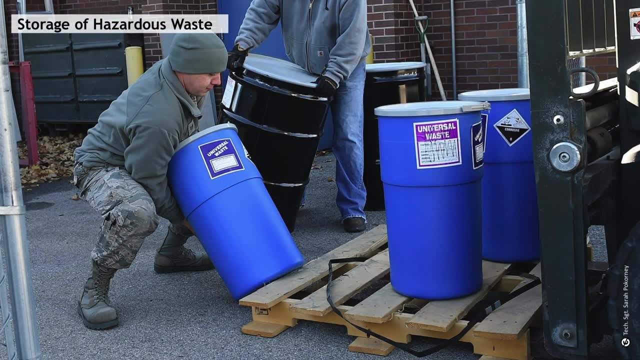 content, physical state, date of first and last deposition, amounts and codes of hazard category. These containers must be kept in good condition and close to or covered in order to avoid leaks or damage and to protect them from weather. If hazardous waste is transported, generators should partner with. 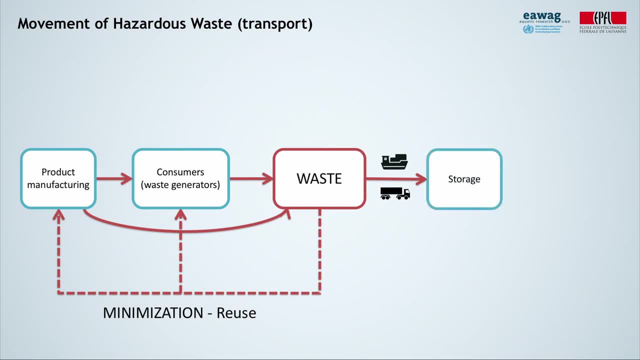 authorized collectors to collect their waste. If such waste will cross borders from one country to another, it should be reported to the Basel Convention Secretariat. as explained in the Convention, The environmentally sound management of hazardous waste consists of several steps. First, the materials go through a pre-processing stage where the hazardous elements are. 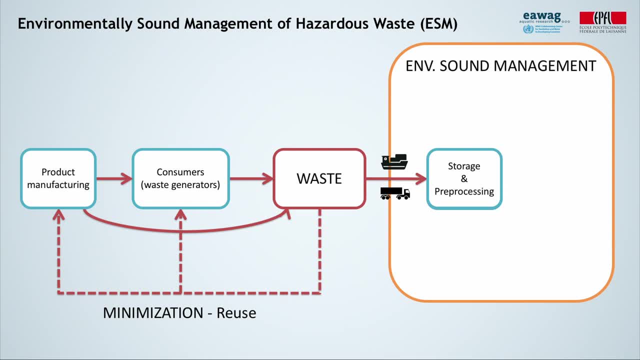 either separated, immobilized or degraded. These methods can be classified into physical, chemical, thermochemical and bioremediation methods. Then these materials can be stored again until they are either recycled, processed through other recovery options, such as energy recovery, or finally disposed of.